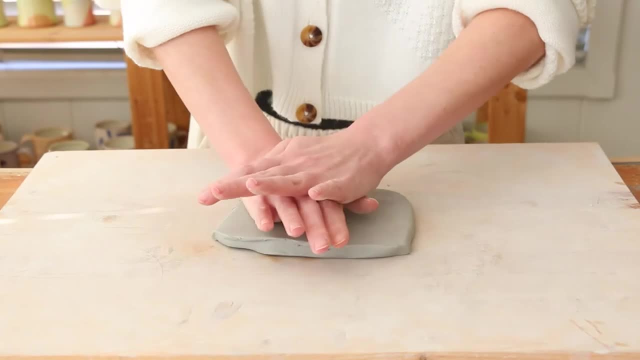 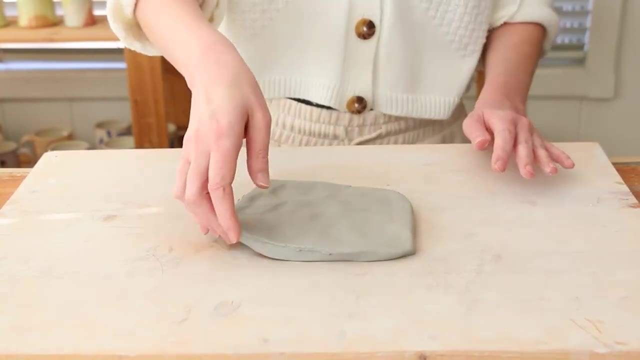 So I'm just going to press, press, flip until I get to that thickness that I'm looking for Again, about a thickness of a pancake, Or, if you want to be more technical, it's like closer to like one quarter of an inch plus a. 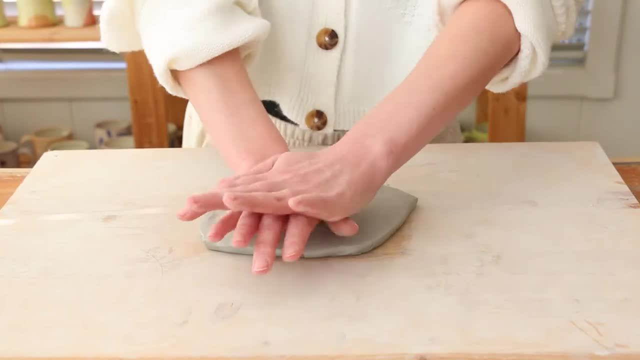 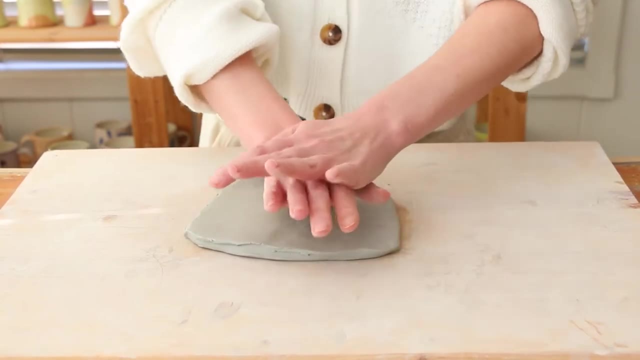 little bit Like one quarter of an inch is kind of what we're wanting in the final final product after we use the rolling pin. So right now we're kind of trying to get like close to that, if that makes sense. One thing to look out for if you're making a slab like this just completely manually is: 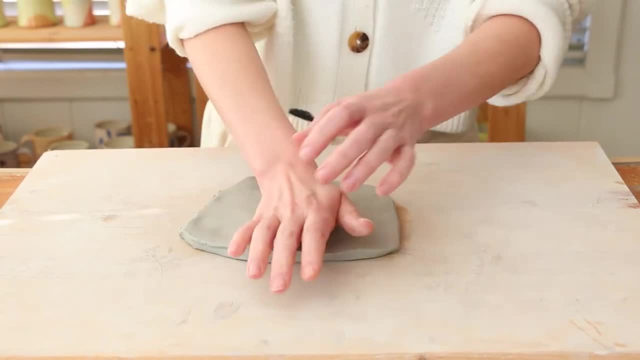 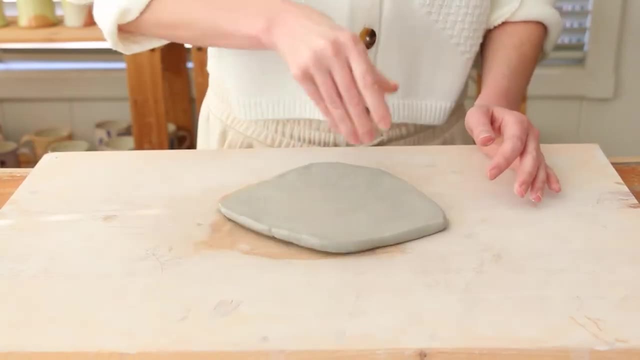 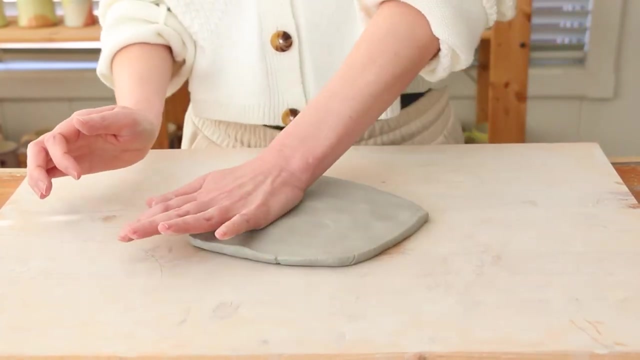 a lot of times folks get a thicker spot in the middle because, for whatever reason, we just don't attend to that part of the slab as much. So make sure that you're not putting extra pressure on the edges and leaving the middle kind of unattended. Okay, I think that looks pretty good to go ahead. 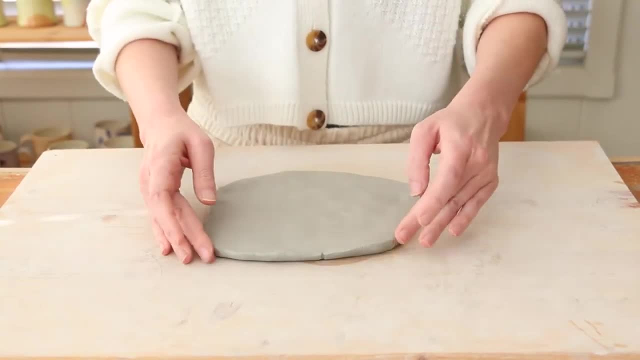 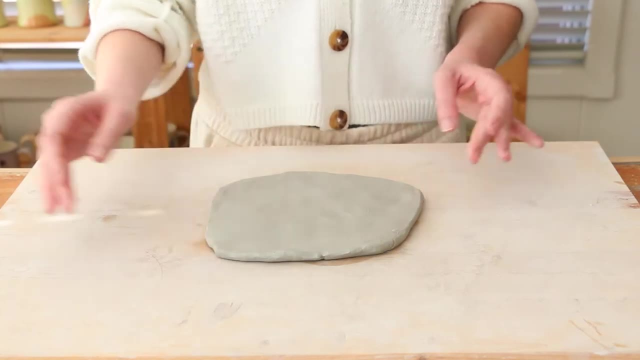 and go in with the rolling pin can see I got most of my size and my kind of my thinning done with my hand. The rolling pin is not really for that part. The rolling pin really helps us more with refining and getting the last little. 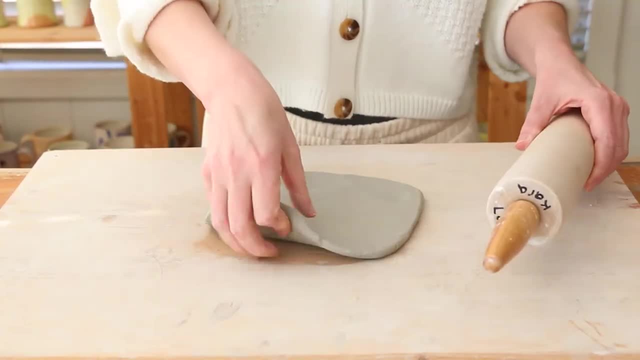 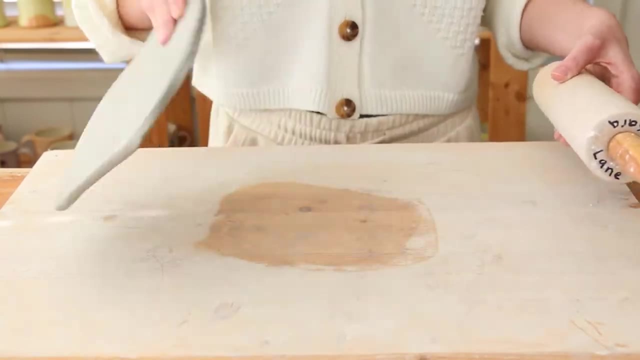 bit of size out of it that we can get. And I'm just going to kind of do this quickly, friends. but if you want to see a little bit more detailed tutorial about just this part- just making the slab- we do have a video about that. 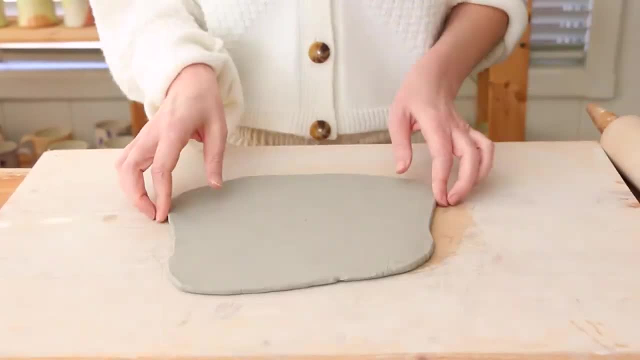 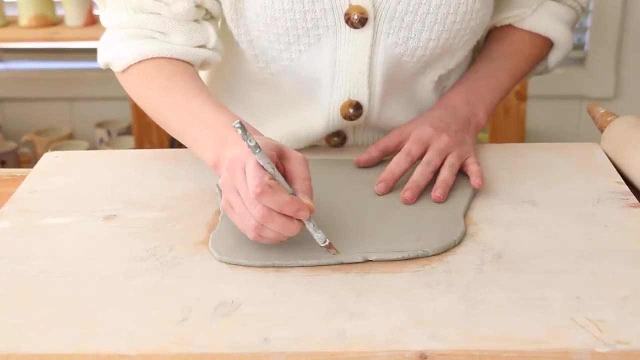 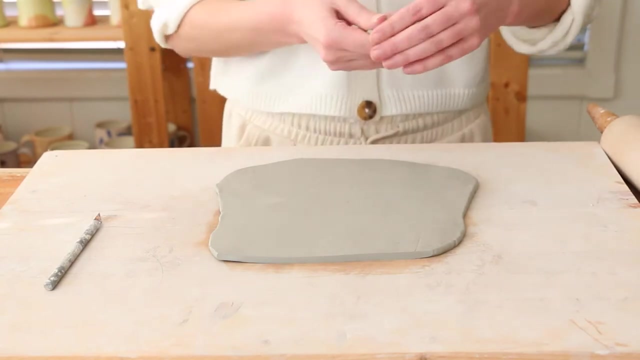 All right, So that's looking pretty good. but I always like to just cut off a little piece of crust so I can check the thickness of my slab, truly see what it's looking like on the inside, And I think that's looking pretty good. Okay, So now what we're going to do is I'm going to use 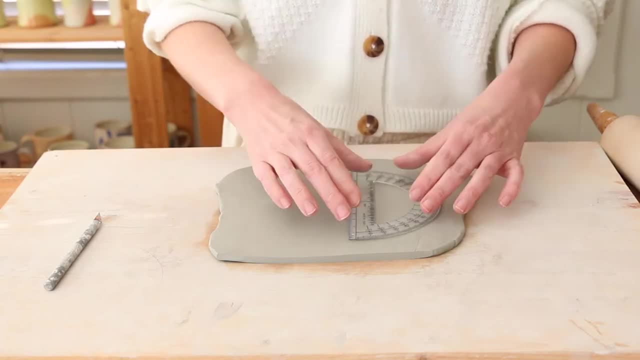 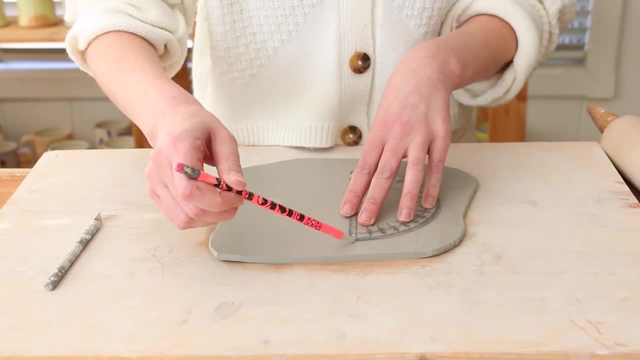 this tool to create a circle shape, because I want to make my plate or my dish into a circular shape. But the nice thing about this project is you could do any shape that you want that fits on the slab, So you don't have to do just. 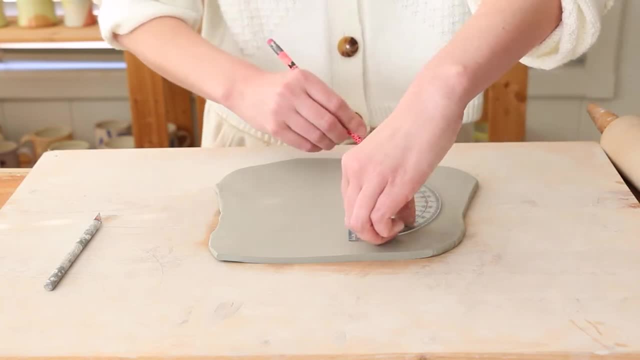 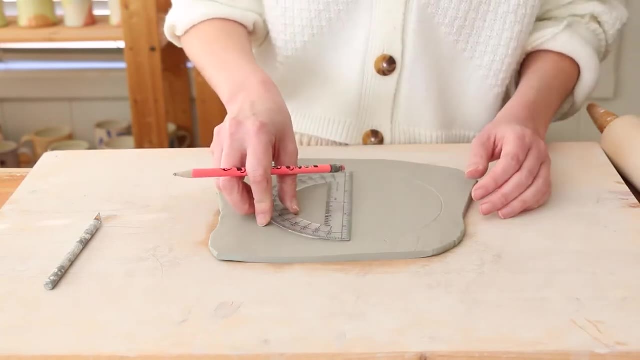 like a geometric shape like what I'm doing, Like you could do a circle, square, triangle, rectangle, dish- any of those things work, but you can also do organic shapes or like non-symmetrical shapes. The only things that don't work very well that I've noticed is like 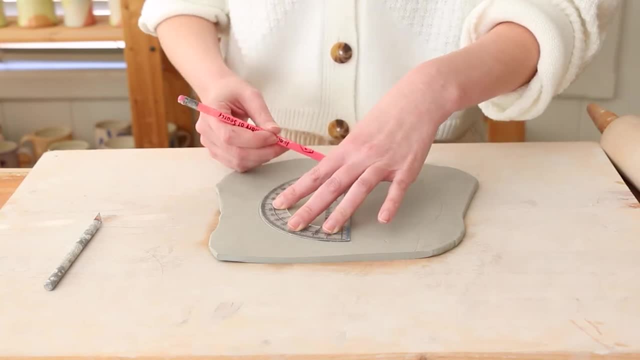 a star shape, a sun shape, anything that has like protruding, like little parts that stay in place. So I'm going to do that, And then I'm going to do a little bit of this with my table tool, And then I'm going to keep the texture in place And then I'm going 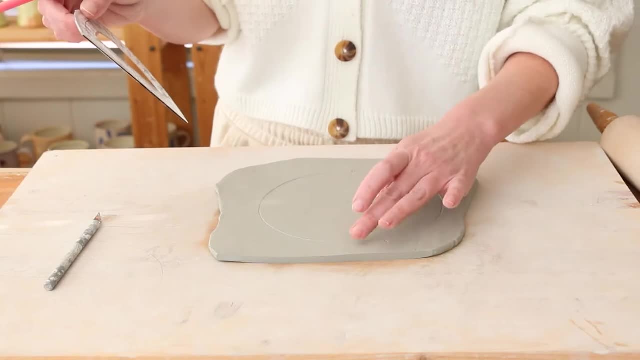 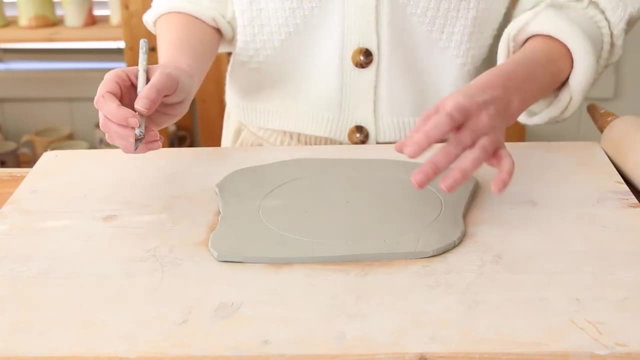 to stick off of it. That can get kind of challenging to do, to create the rim of the dish on a shape like that, And it'll make more sense what I mean here in just a minute. but other than those kinds of shapes, really anything will work for this, and organic shapes are really. 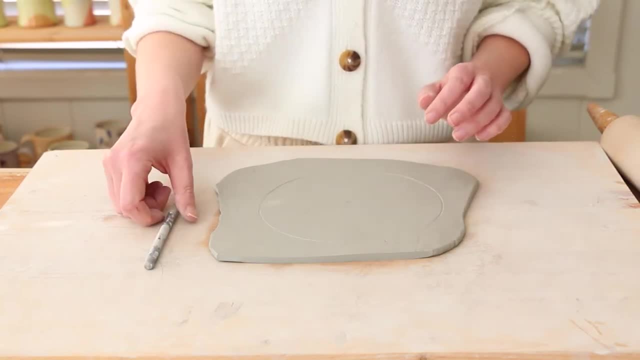 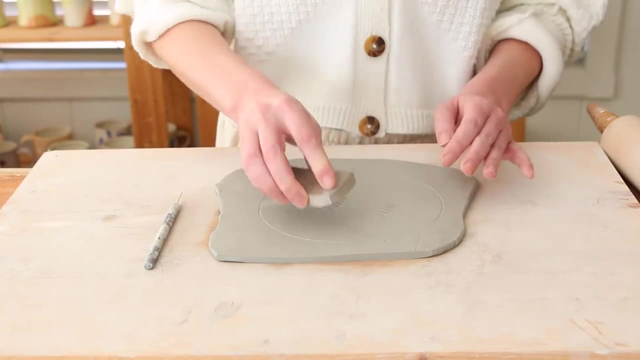 cool for this project too, but I'm just going to stick with my circle for today. So now that I've got that laid out, I'm going to add some texture to it, and you could do this with texturing plates where you can stick it on the other side of the dish And then you guys have a little bit of the slim. 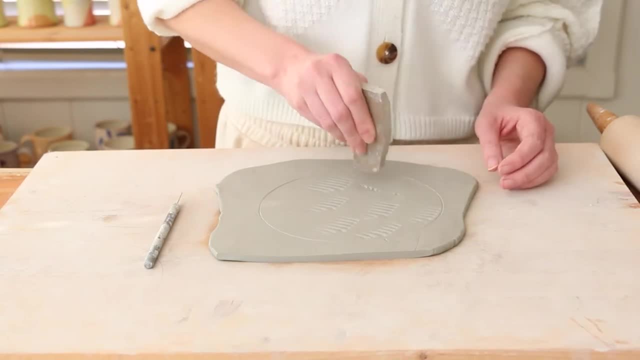 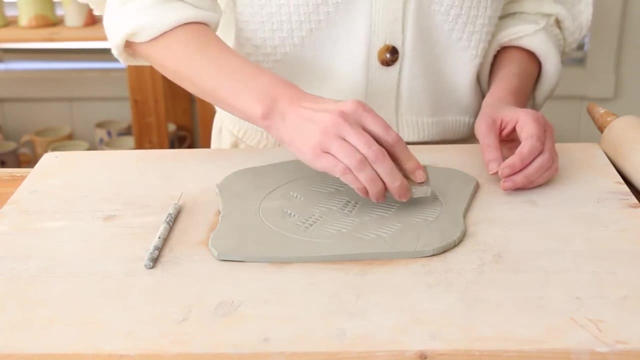 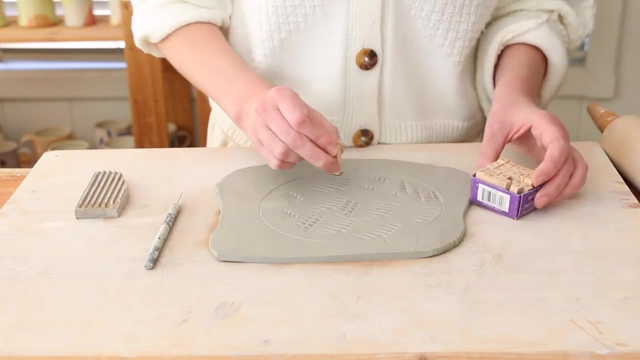 you, um, you roll those into the surface of the clay with your rolling pin or just with your hands. You can use stamps, you can use a dull pencil- really anything that you want will work here. I also like to use my letter stamps just as like decoration. I just think that's fun to do. 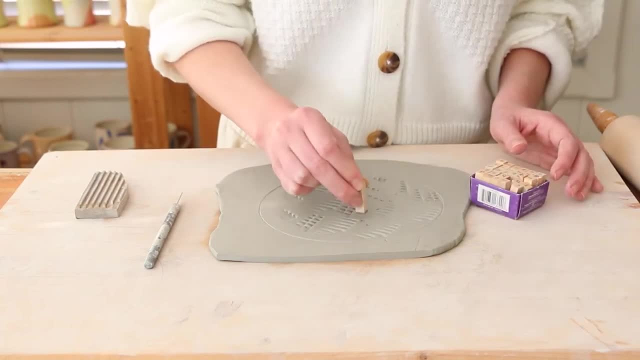 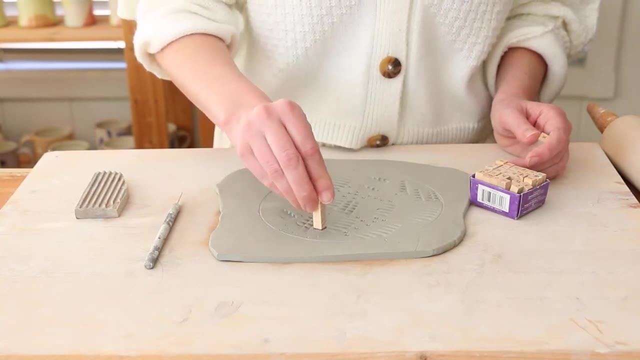 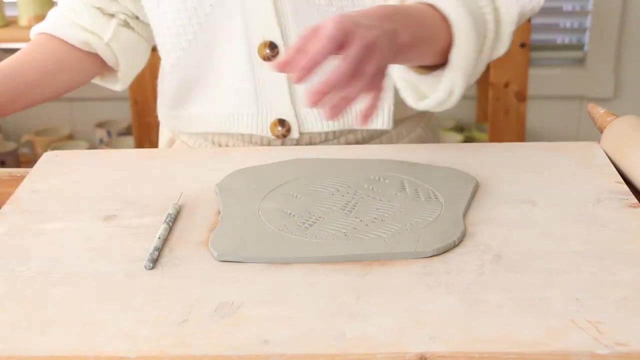 sometimes. So we'll just pop a few of those on the surface just for fun, and, again, feel free to decorate it however you want. That part is completely artist's choice. Okay, so now we've got a little interest going on in the surface, We're going to cut this guy out using an exacto. 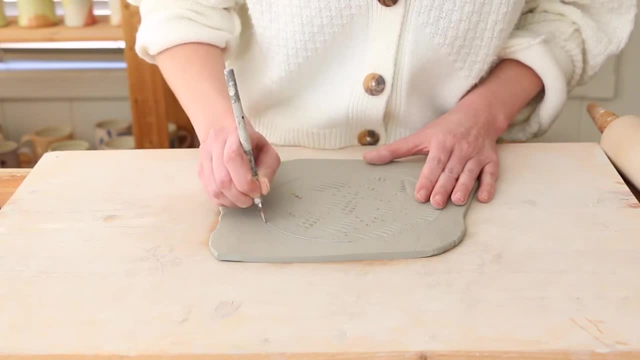 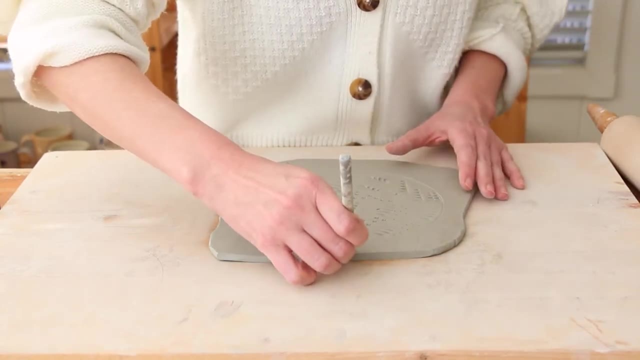 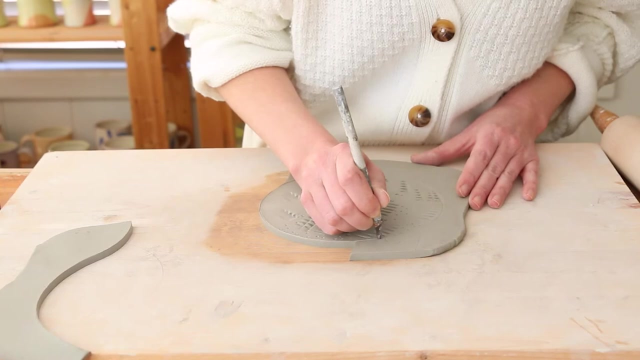 knife and holding it really straight up. It's easy to get your knife leaned to the side and then you end up with an angled edge, which isn't the end of the world. but if you can avoid it, you would want to try. I also always tell my students: cut the edges off in pieces like this: 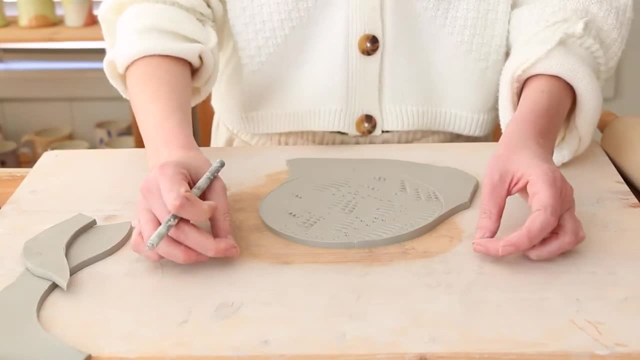 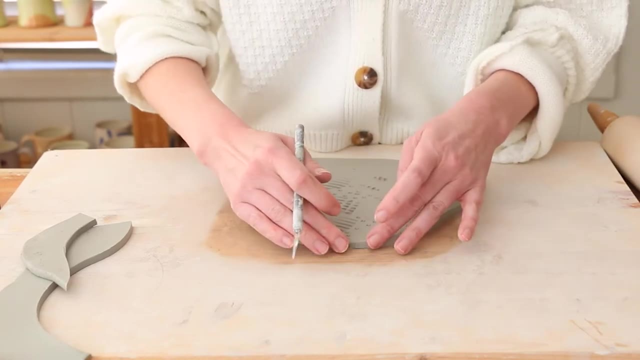 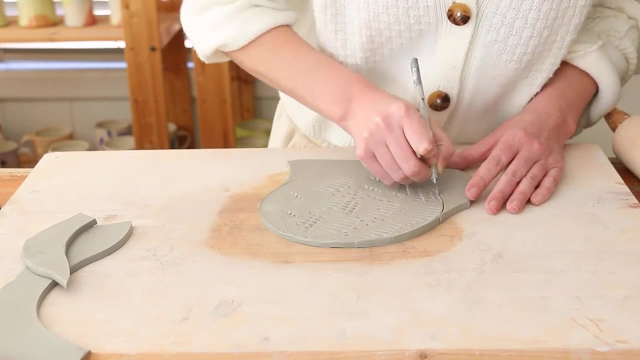 because sometimes if you go all the way around, then when you lift the edges off it takes your dish with it and it can bend it back and like. the main optimum goal with a slab is to keep it flat and straight at all times. so then you don't have kinks in your clay that cause problems as it's drying. 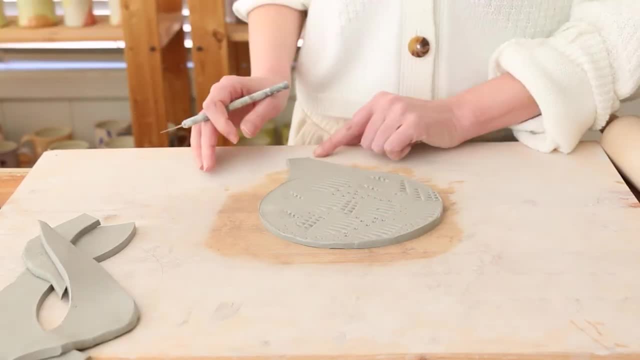 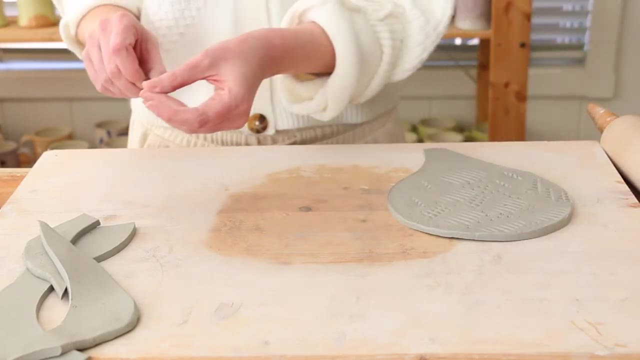 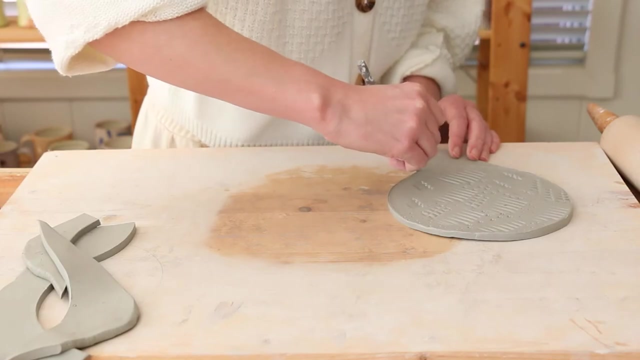 All right, so I'm just going to finish cutting This out. well, I have this little bit here. I'm actually going to use that as like a tab to gently lift this and move it onto a dryer spot. Okay, just finish up that last little cut. there we go. 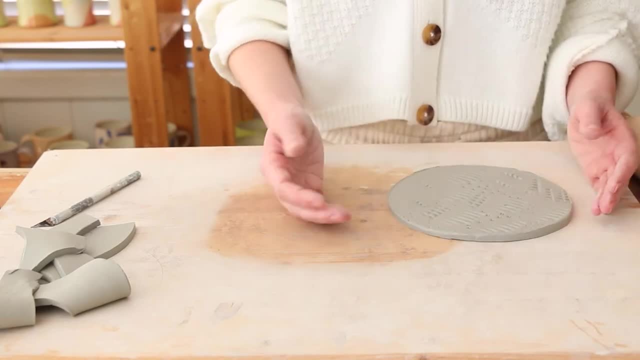 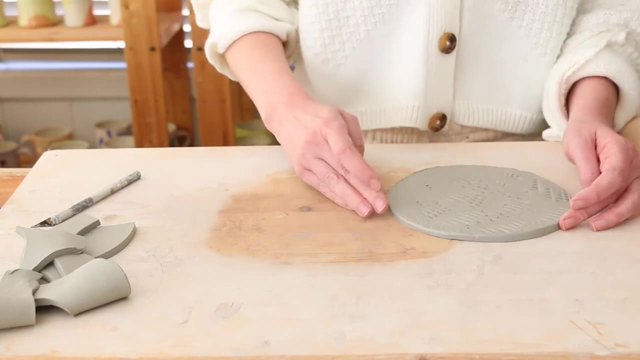 So what we have now is just a flat piece, and all we're going to do to complete this is just flip up the edges to make a rim. So that really takes this from just kind of a flat, non-descript piece that you're not really sure what it is, and it makes it really clear what the 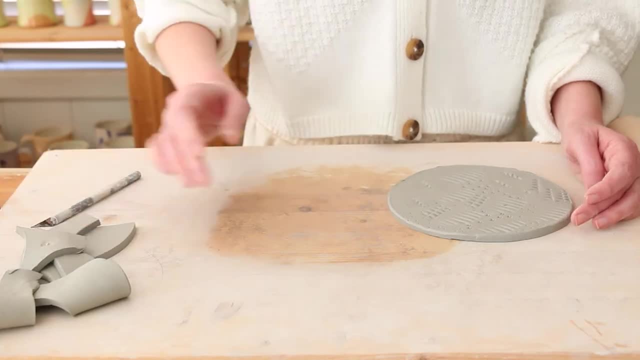 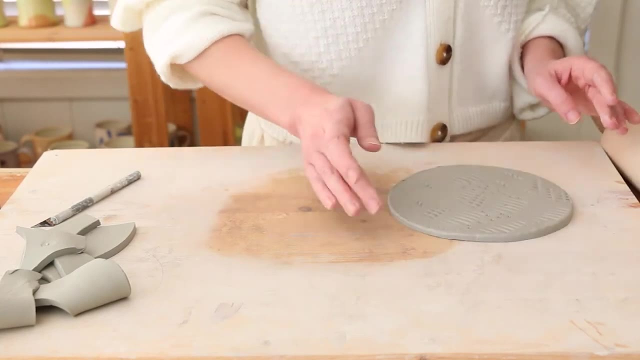 purpose of it is because whenever you make a plate, the rim, you know, or the edge is what kind of indicates what you're supposed to do with that piece. So before I do that, I'm just going to sort of pat these edges down, get them a little more rounded, and you could do this with like a barely 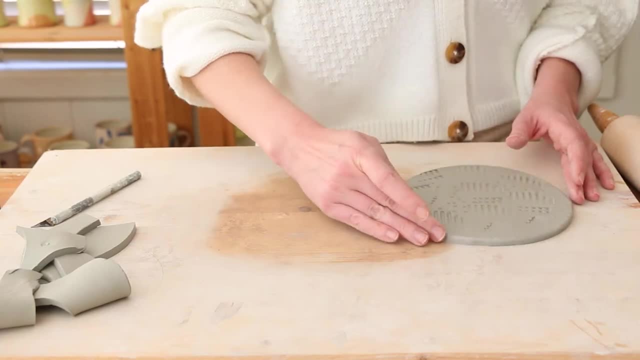 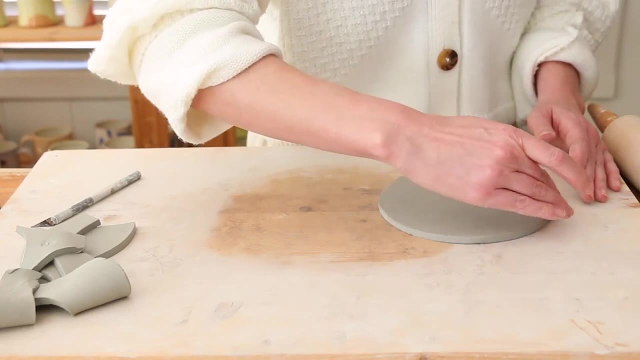 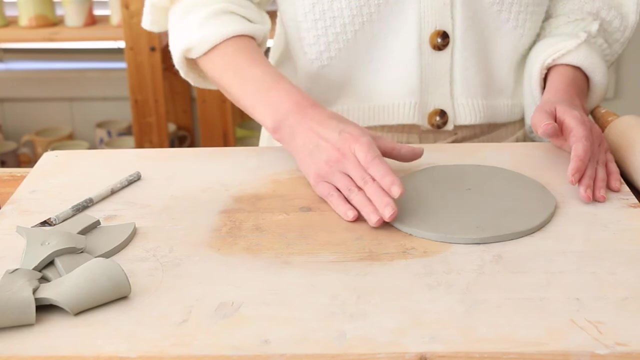 damp sponge. Kind of do this part however you want. I've just kind of developed this little tapping That I like to do because it just sort of pushes down that hard angular edge and it doesn't rub and pull like the little, doesn't create the little crumblies. 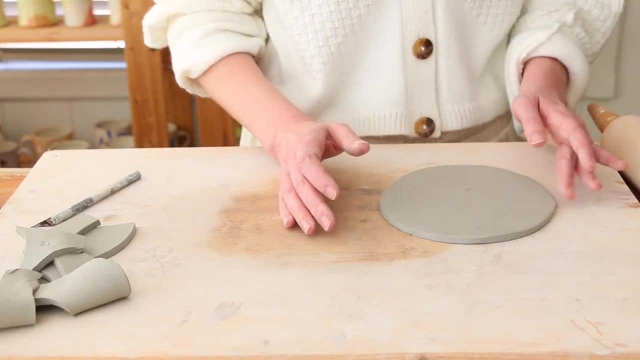 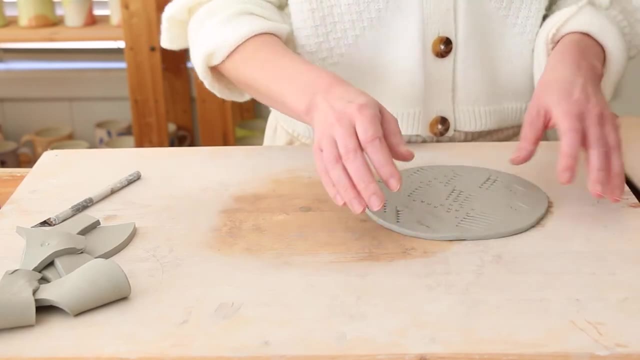 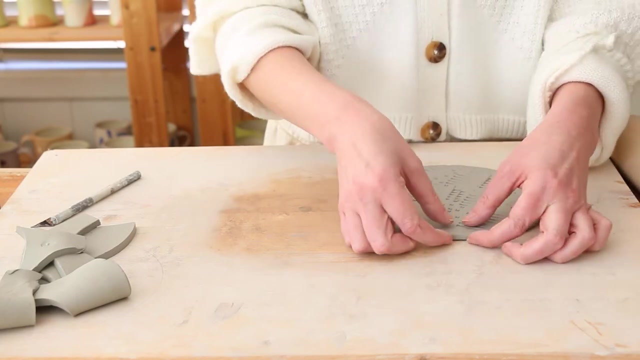 or like the little scraps that you sometimes get from dragging your finger across the surface. Okay, that's pretty good. alright, So now for like the magic. So what I'm going to do here is I'm going to turn this edge and I'm going to point this, this side part. I'm going to 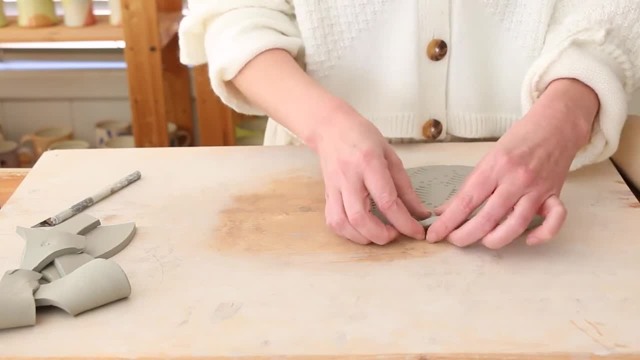 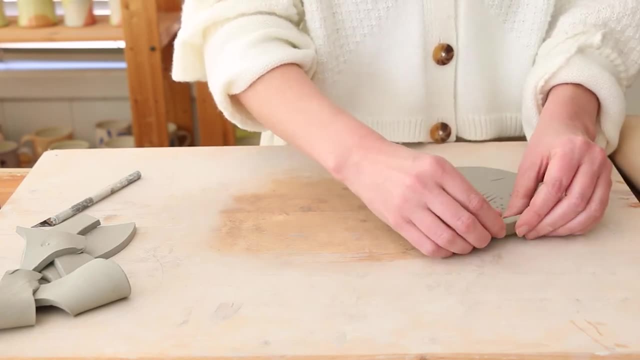 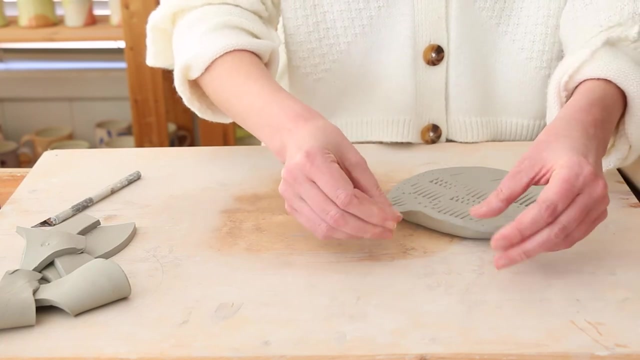 to try to point it towards the ceiling. So a lot of times, what people do here, though, is they pinch to get it up, and what you want? you want to avoid pinching and be like turning or bending instead, So it's kind of like this rather than this, So it takes a few. it usually takes me a few rounds to. 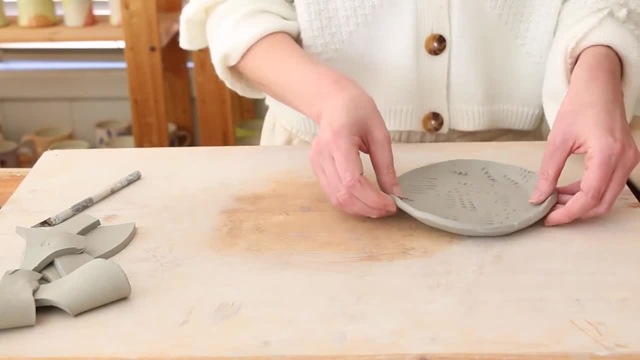 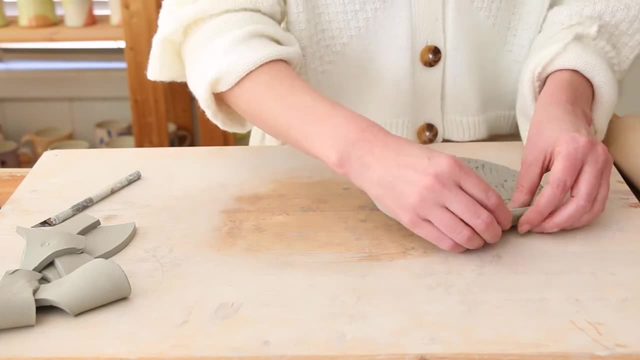 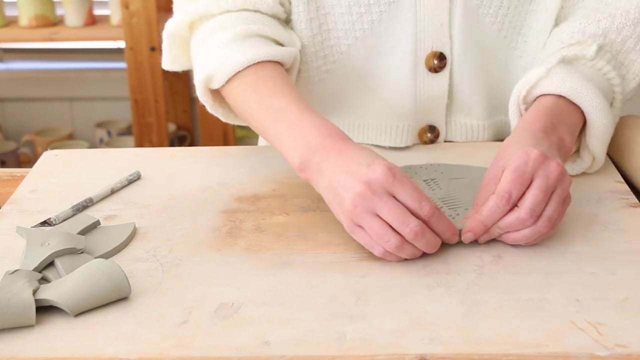 go around the tray to get the edge like crisp enough for my my liking. So it's not just like a one shot thing where you do it once and then you have to stop. You can fiddle around with it as much as you like and define that rim as much as you like. So now what I'm doing is I'm kind of bending.